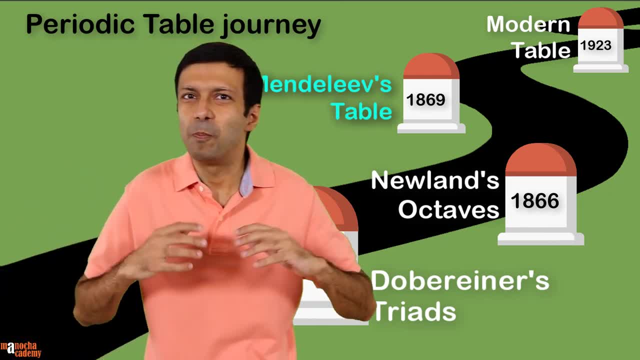 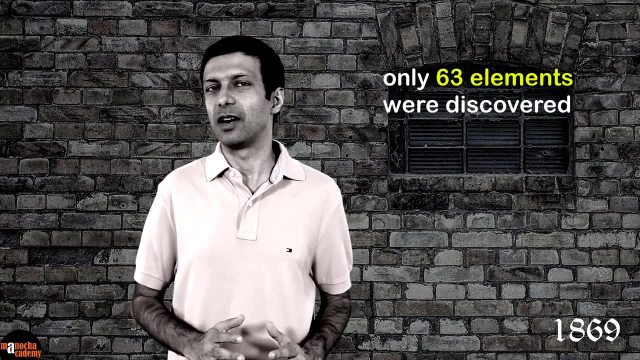 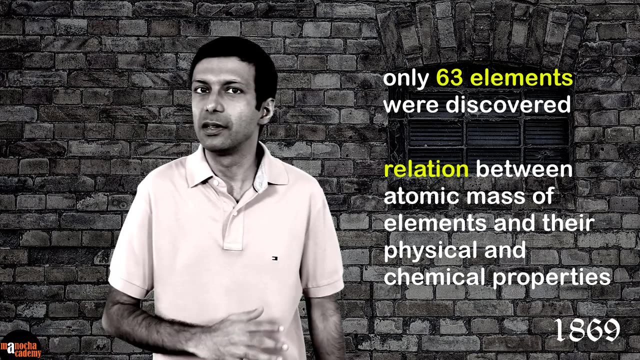 from the modern periodic table. So let's go back to Mendeleev's time. Imagine we are in 1869.. Only 63 elements were discovered at that time And Mendeleev was looking at the relation between atomic mass of elements and their physical and chemical properties. So let's discuss. 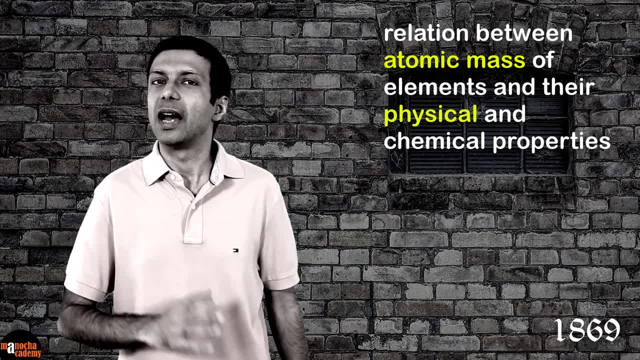 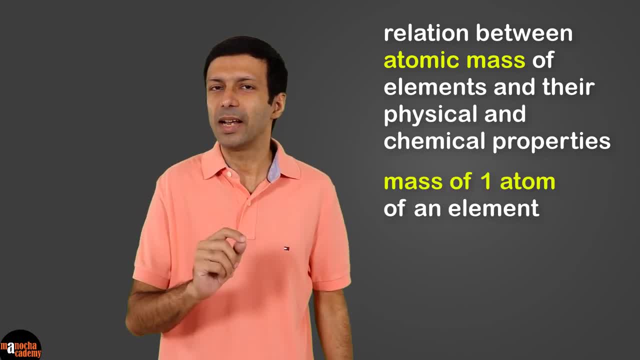 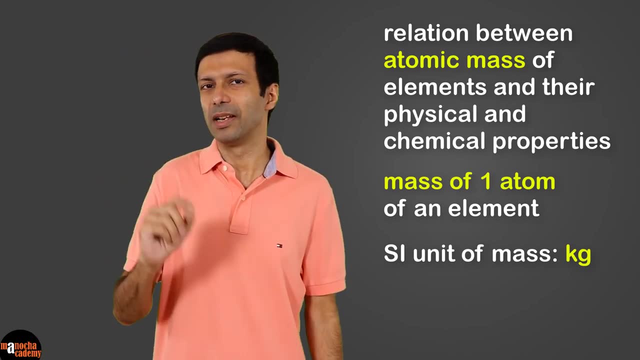 these three things: atomic mass, physical and chemical properties. What is atomic mass? That simple: the mass of one atom, of an element. The SI unit of mass is kg, But since the atom is really small and light, a more convenient unit called atomic. 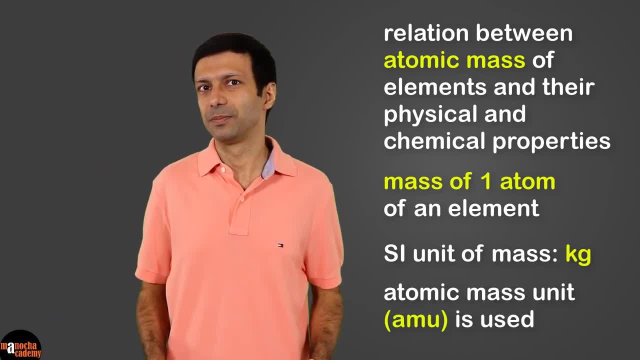 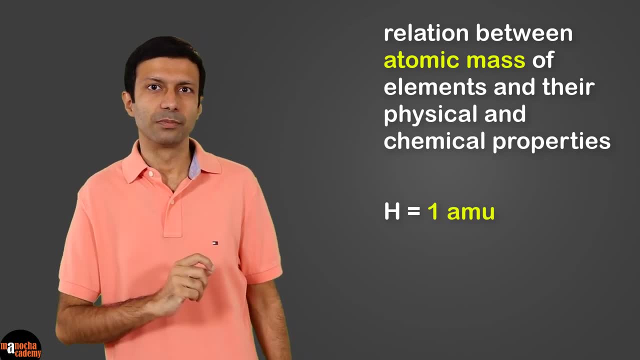 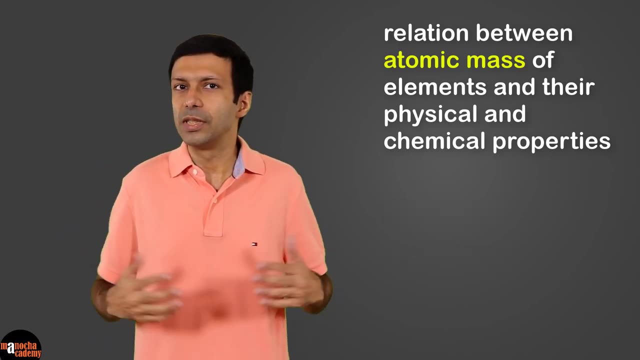 mass unit, or AMU in short, is used. Let's take some examples: Hydrogen has an atomic mass of approximately 1 AMU, And carbon has an atomic mass of approximately 12 AMU. Now let's talk about physical properties. So what are physical properties of an element? 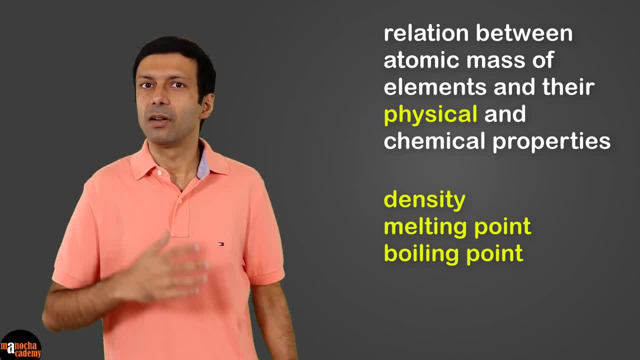 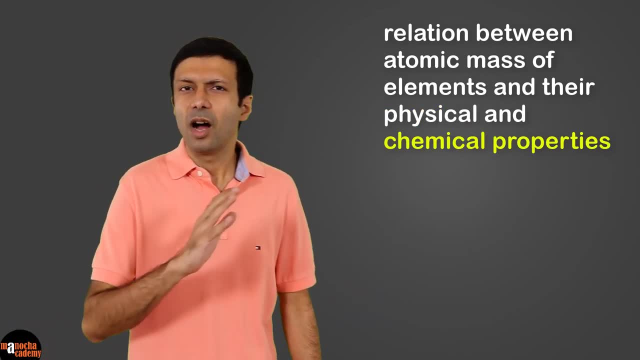 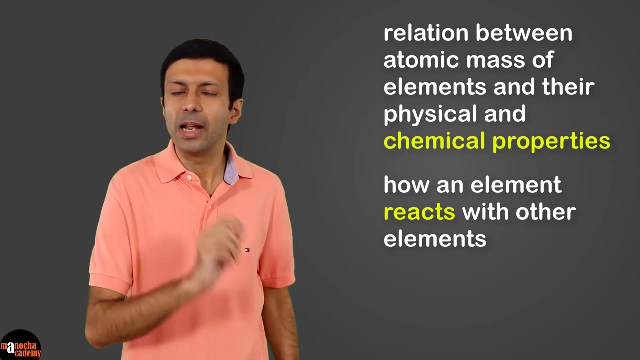 That's right. things like density, melting point, boiling point of the element. What are chemical properties of an element? Chemical properties are how an element is react with other elements. To look at this in a systematic way, Mendeleev looked at how an element reacts with hydrogen. 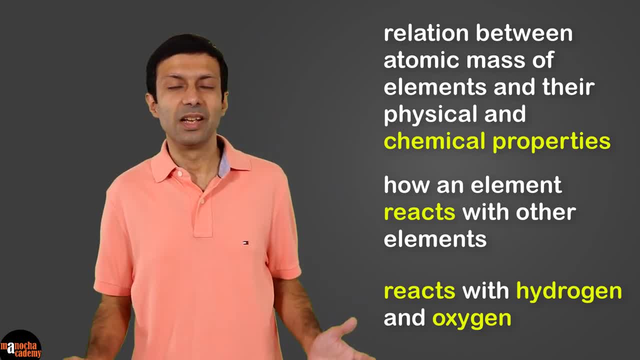 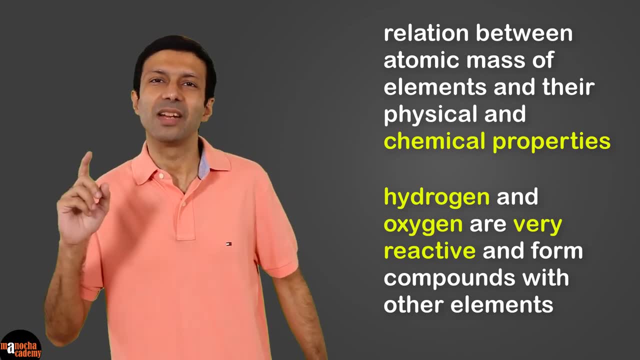 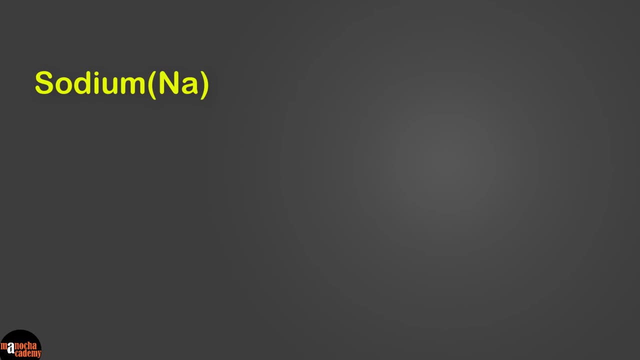 and oxygen. He chose hydrogen and oxygen since they are very reactive and form compounds with other elements. Now let's understand this with a couple of examples. Let's take the example of sodium. The compounds formed with hydrogen and oxygen are sodium hydride. 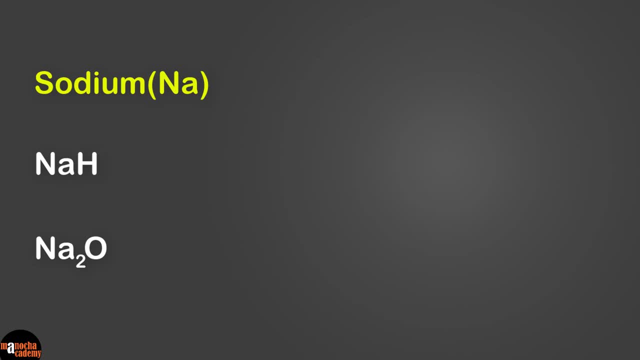 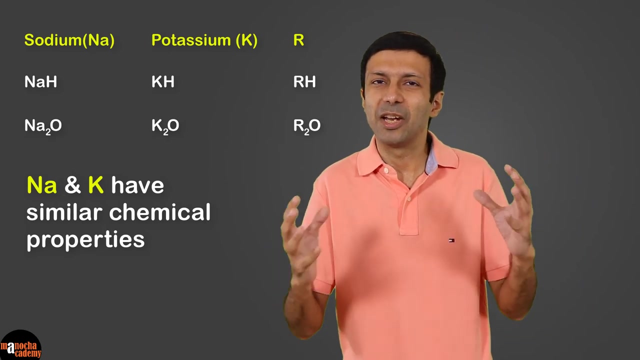 NaH and sodium oxide, Na2O. Similarly for potassium, the compounds formed are KH and K2O. If we represent the element as R, then the chemical formula is same for both RH and R2O. So sodium and potassium have similar chemical properties and can be grouped together. 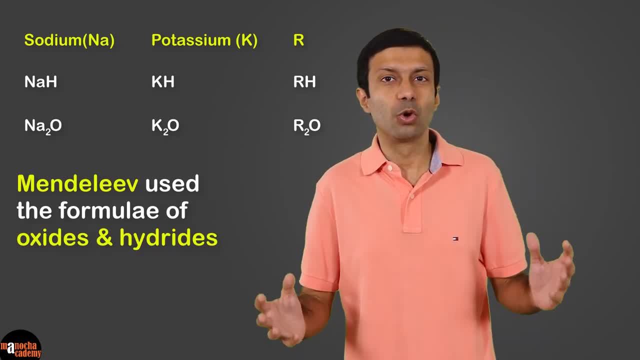 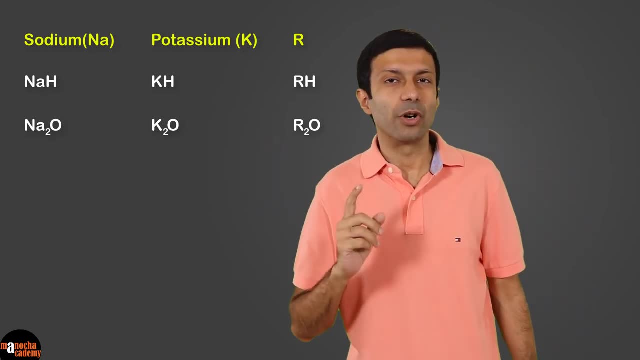 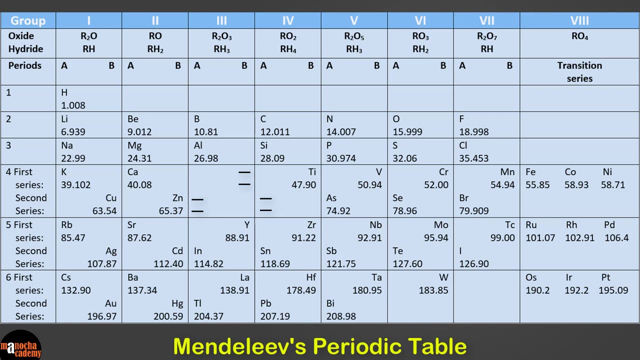 Mendeleev used the formula of oxides and hydrides to group the elements together. So if you look at the top row in Mendeleev's periodic table, you will see this formula for each group. Mendeleev's periodic table looked something like this: As you can see for group 1, the 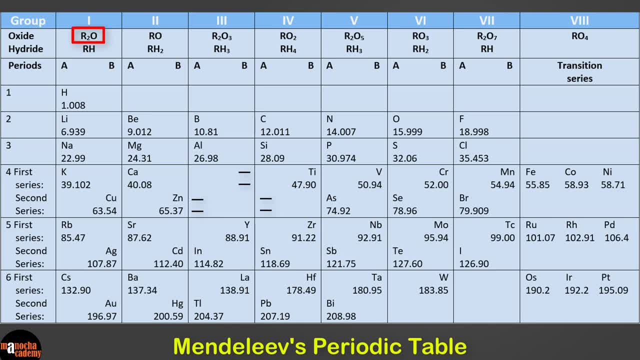 oxide formula is R2O and hydride is RH. For group 2, the oxide is RO and hydride is RH2, and so on. Elements were mostly arranged in order of H2O and H2O For group 2, the oxide. 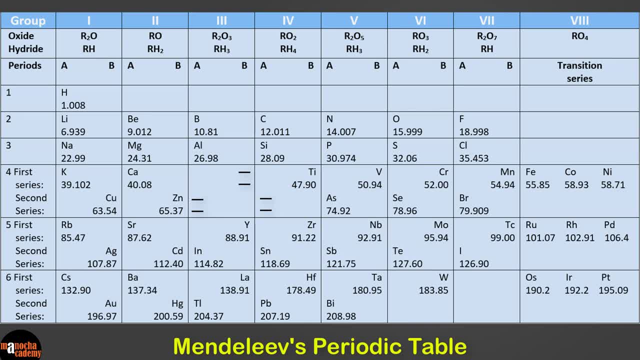 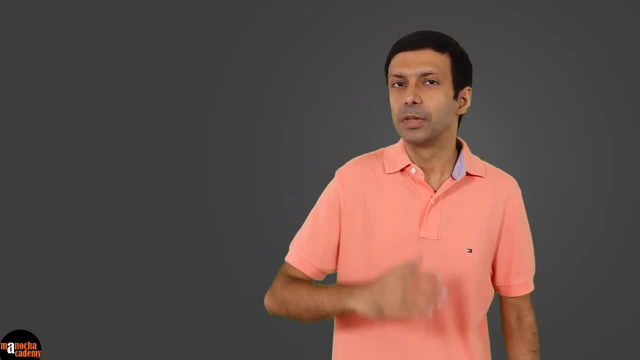 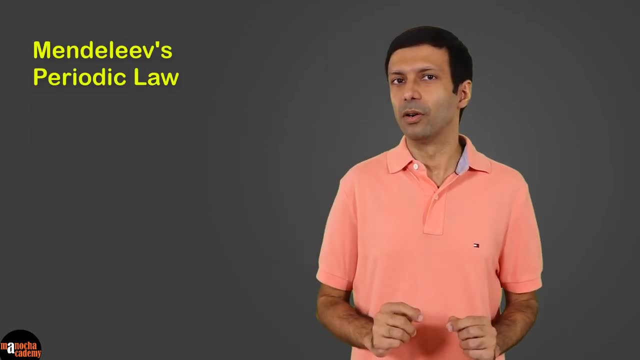 was arranged in order of increasing atomic mass. The horizontal rows are called periods and the vertical columns are called groups. Mendeleev observed a repetition in physical and chemical properties. He formulated Mendeleev's periodic law, which states that the properties of elements are periodic function of their 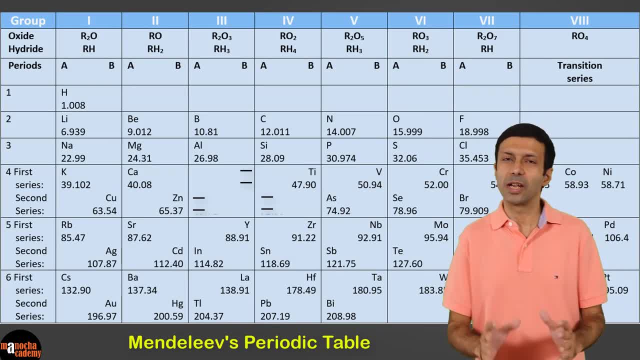 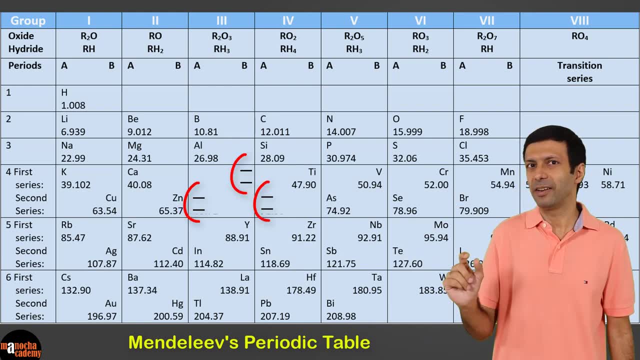 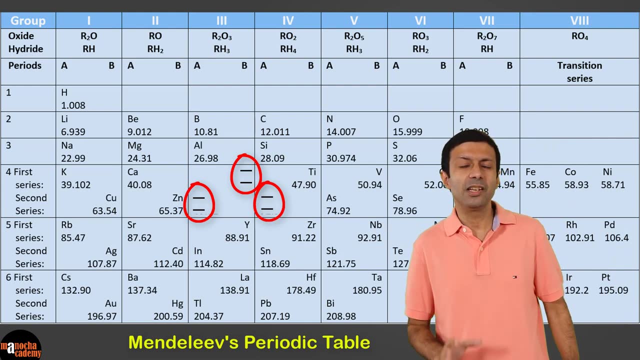 atomic masses. Now, if you closely look at Mendeleev's periodic table, you will find something really interesting. Do you see some gaps in there? This was the genius of Mendeleev, This was his sheer brilliance, Because he didn't forcefully try to fit the elements. 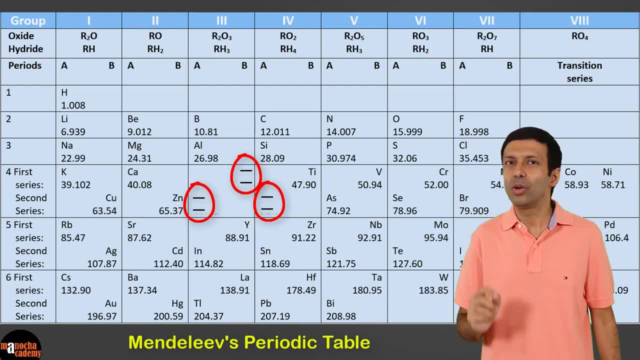 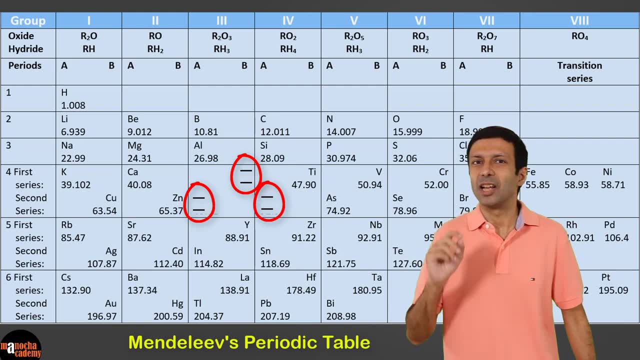 into his table. Remember, at that time only 63 elements were discovered. So he left gaps and boldly predicted that we haven't discovered these elements yet. Mendeleev even gave names to these elements. For example, he called the element in this gap as eka-aluminium- Eka is the Sanskrit word. 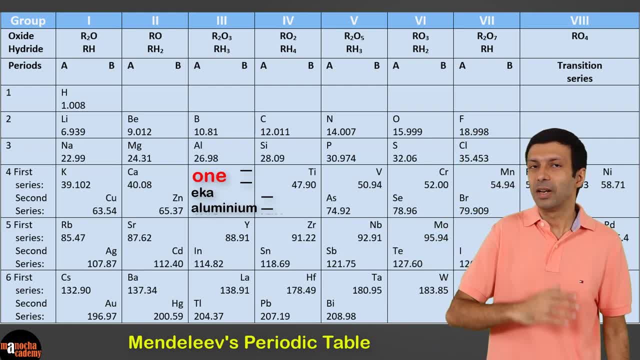 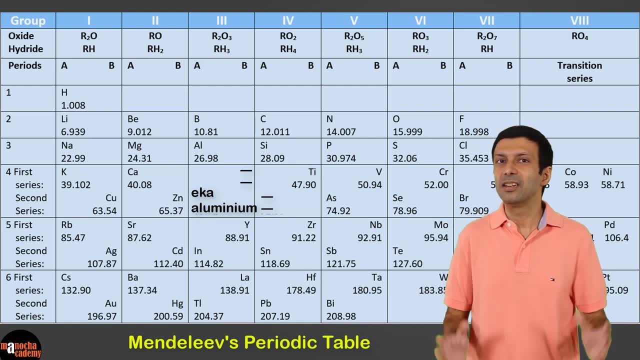 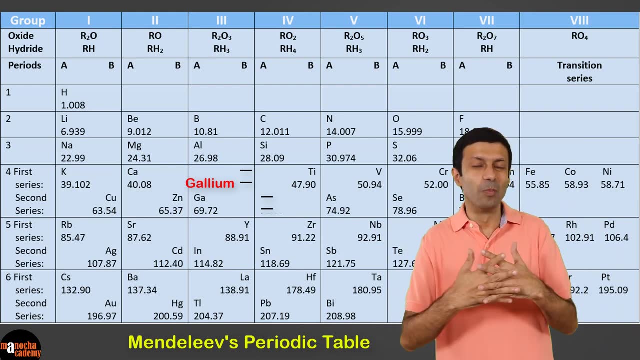 for one. So first comes aluminium and then this unknown element. He predicted the properties of eka-aluminium And many years later an element was discovered. It was called gallium, And guess what? The properties almost matched. Actually, he gave names to other elements such as eka-boron, eka-silicon. Many years, 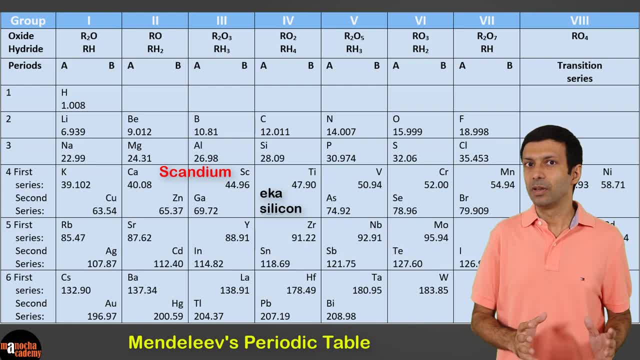 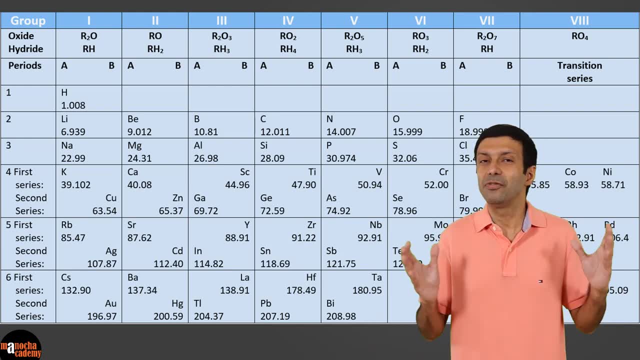 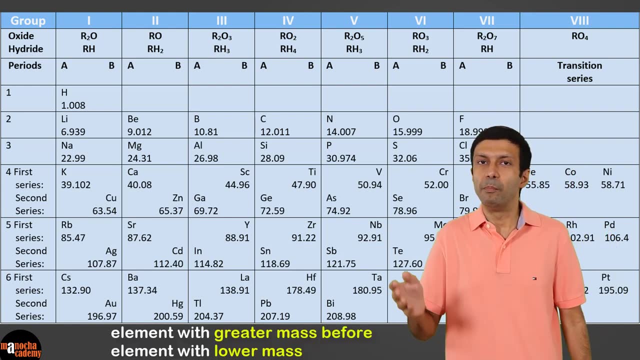 later these were discovered and named scandium and germanium. This was Mendeleev's greatest achievement. Another interesting thing Mendeleev did in his periodic table is: in some cases he placed an element with slightly greater atomic mass before an element with slightly lower atomic. mass. He did this so that elements have a slightly greater atomic mass than the elements with a slightly lower atomic mass. So that's why we call them the eka-aluminium elements. So it's an interesting thing. So here is an example of an experiment that Mendeleev did. He did this so that elements have 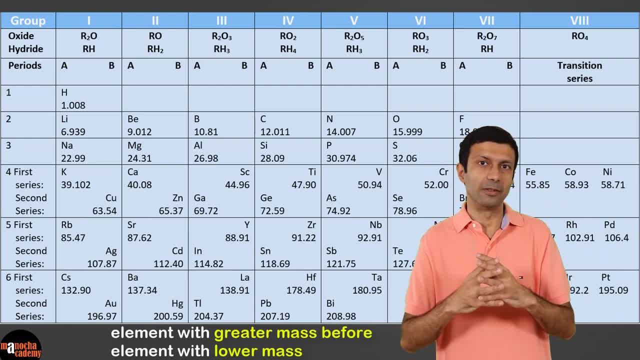 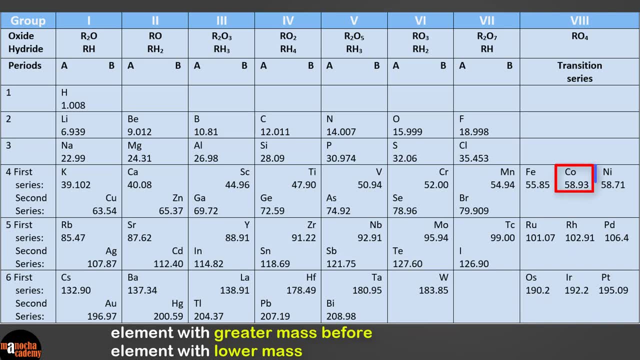 elements having similar chemical properties could be grouped together. For example, as you can see in the table, cobalt has higher atomic mass compared to nickel, So cobalt should come after nickel, But cobalt comes before nickel, since its properties are similar to the elements below it. 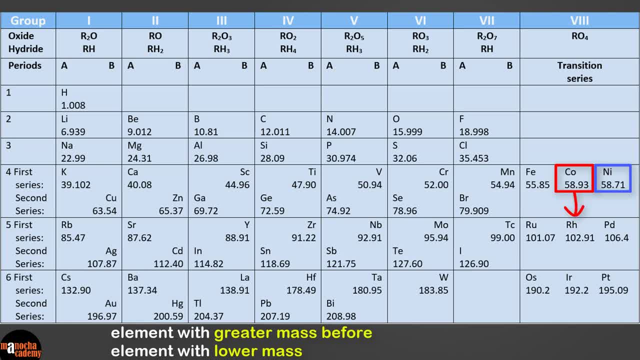 That is, RH rhodium and IR iridium. Nickel's properties are similar to PD palladium and PT platinum, which are below it, So Mendeleev had to make such exceptions where an element with higher atomic mass comes before an element with lower atomic mass. 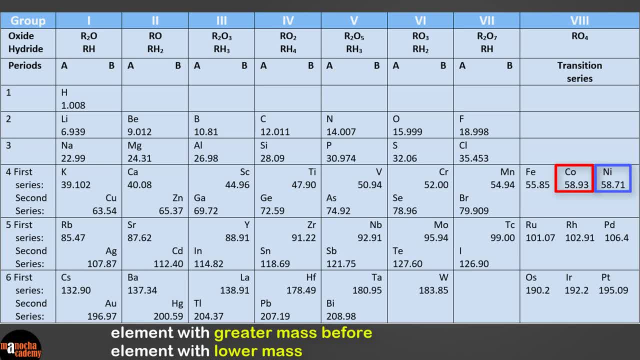 Can you find more exceptions like this? That's right, it's tellurium and iodine. If you look at period 5, group 6 and 7. Can you see that tellurium and iodine? Tellurium which has the symbol Te has a higher atomic mass compared to iodine with the symbol. 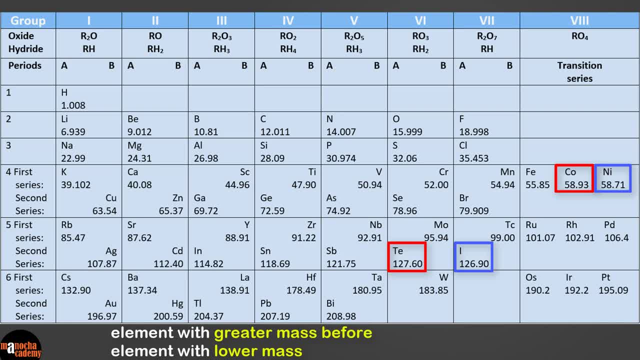 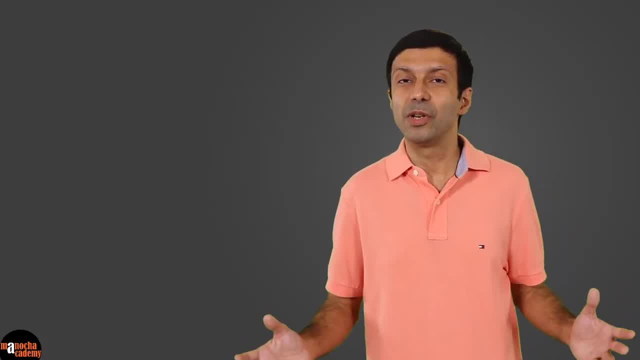 I, But tellurium comes before iodine in Mendeleev's periodic table, So Mendeleev had to make such exceptions. Another achievement of Mendeleev's periodic table was regarding inert or noble gases. Examples of inert gases are helium, neon, argon. 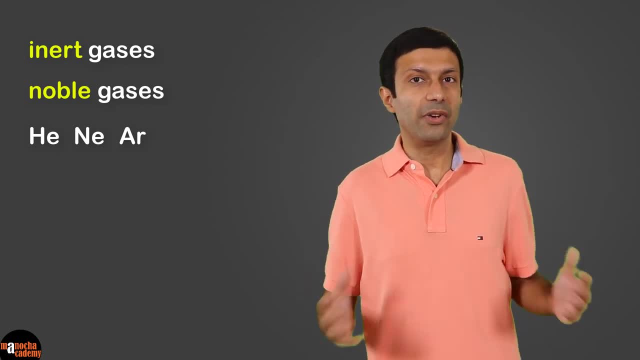 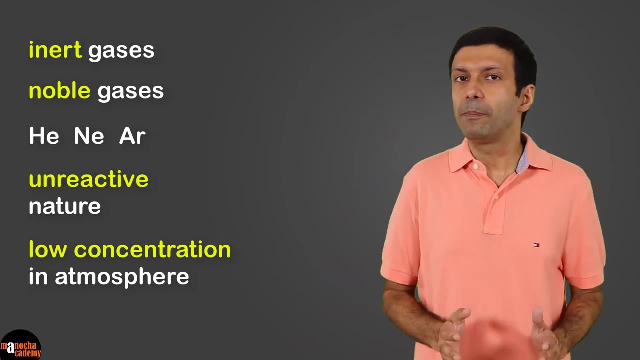 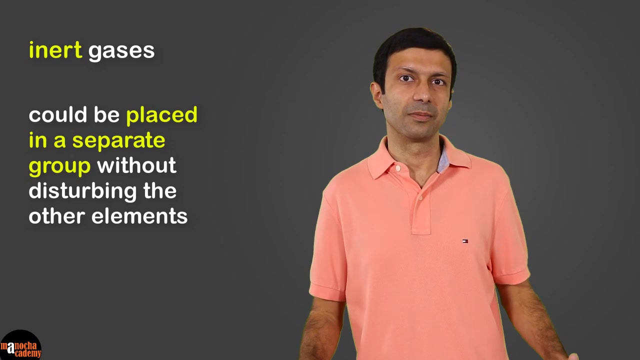 Inert gases were discovered. They were discovered very late because of their unreactive nature and low concentration in the atmosphere. But when they were discovered they could be placed in a separate group in Mendeleev's periodic table without disturbing the rest of the elements. 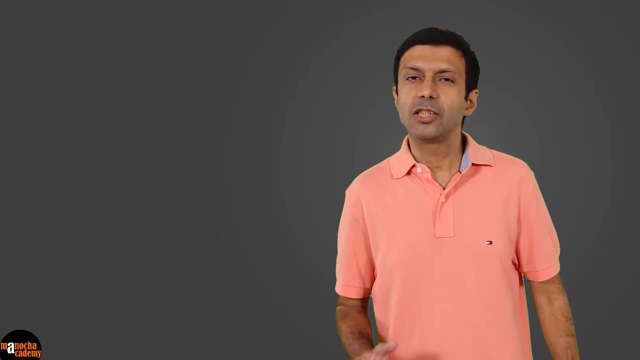 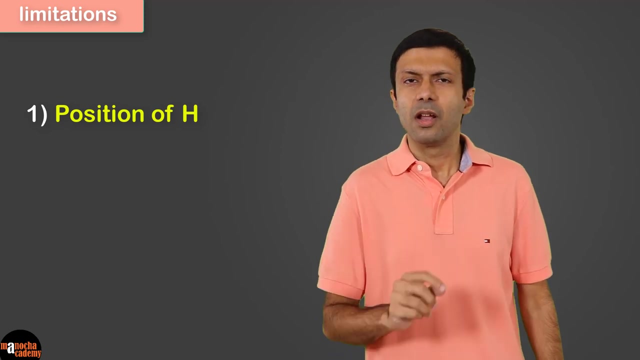 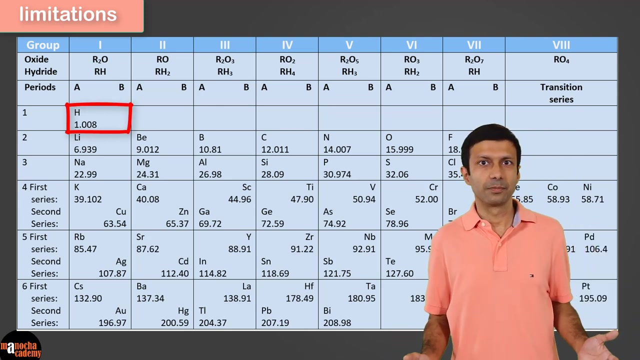 Now that we are done with the achievements of Mendeleev's periodic table, let's look at some of the limitations. The first one is regarding the position of hydrogen. Now, if you look at his periodic table, Hydrogen is in group 1, along with the other alkali metals, because it shows very similar chemical properties. It combines with halogens- oxygen, sulphur- to form compounds having similar formulae. But hydrogen also shows the properties of elements in group 7, which are called halogens. So just like the halogens, it has a diatomic molecule. 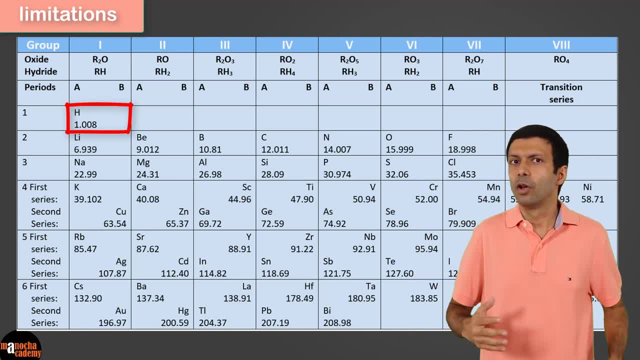 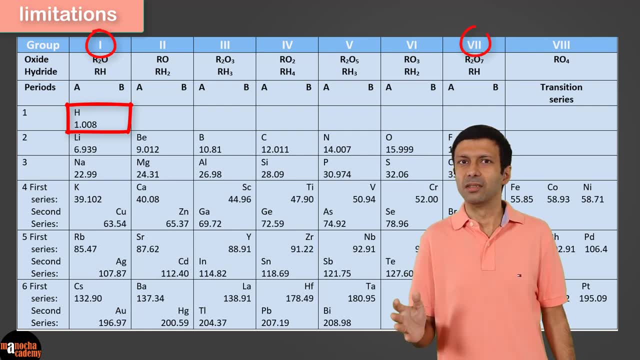 It can combine with metals And with non-metals to form covalent compounds. So where should we put hydrogen? In group 1 or group 7?? So this was the limitation. No fixed position could be given to hydrogen in Mendeleev's periodic table. 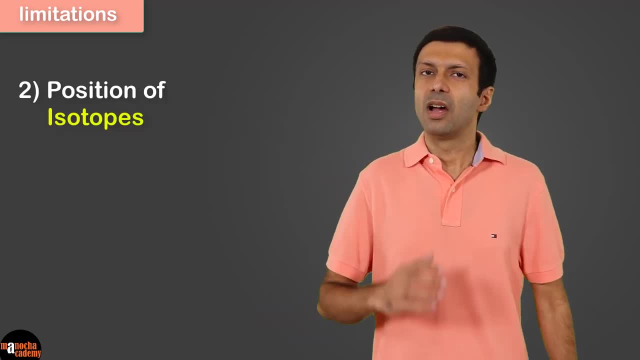 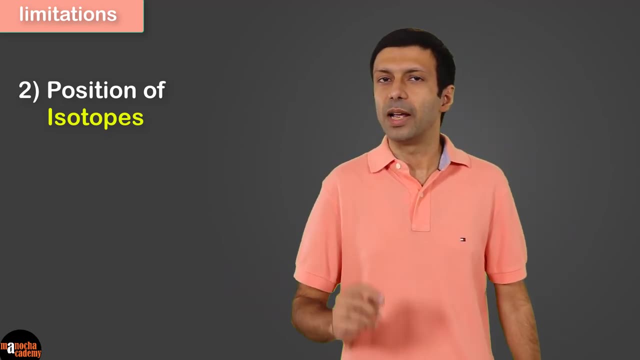 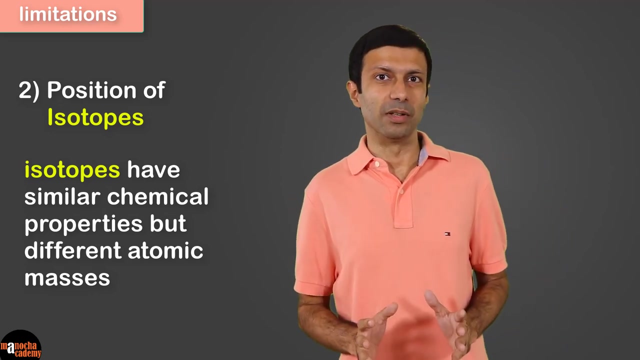 The second limitation was regarding isotopes. Isotopes were discovered much later, after Mendeleev's table was proposed. Since isotopes of an element have similar chemical properties But different atomic masses, they posed a challenge to Mendeleev's table. 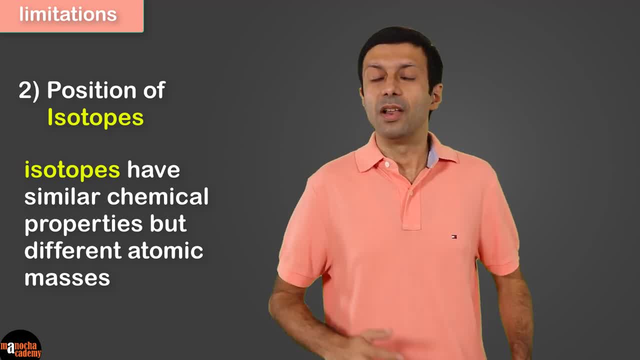 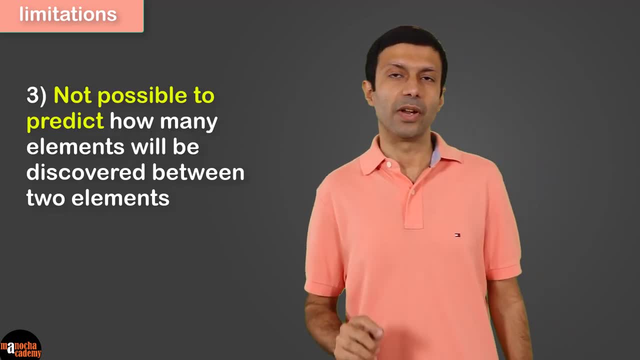 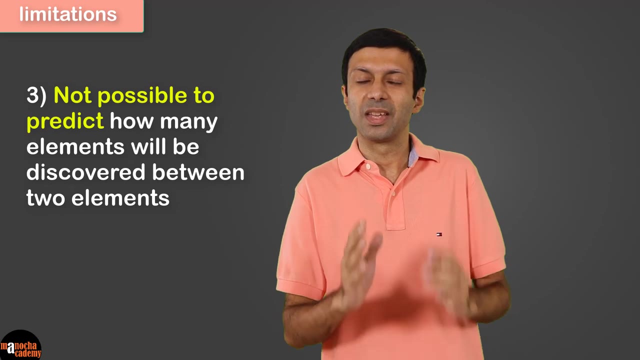 Because we could not fit them in properly. Now let's talk about the third limitation. Since atomic masses of elements do not increase in a regular manner, it's not possible to predict how many elements will be discovered between two elements, And this is especially true for the heavier elements. 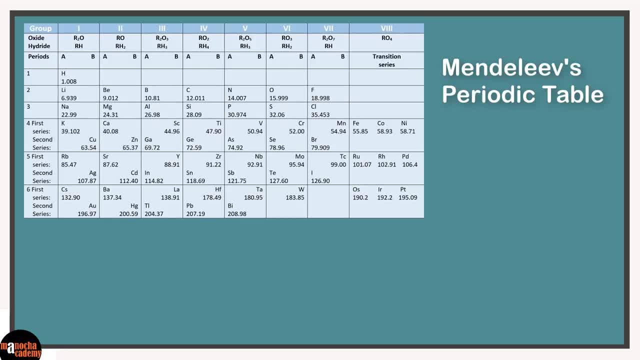 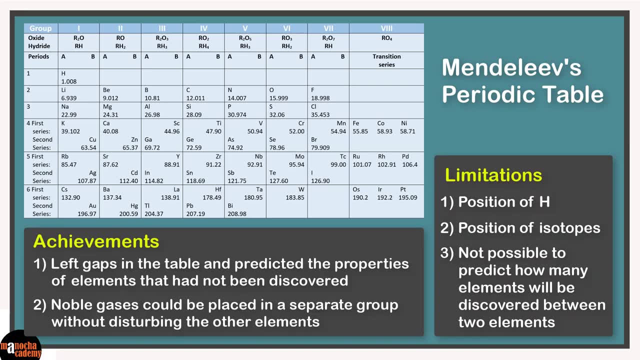 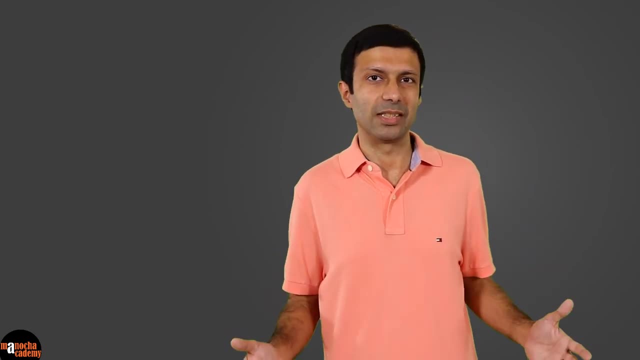 The ones with high atomic mass. So we can place Mendeleev's periodic table on our concept board. Let's also note down the achievements and limitations of Mendeleev's classification. So how were the limitations of Mendeleev's periodic table addressed? 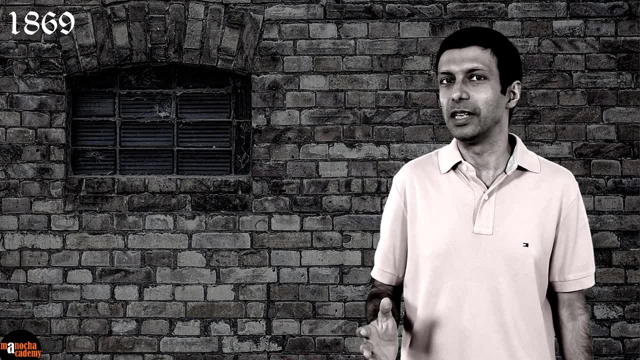 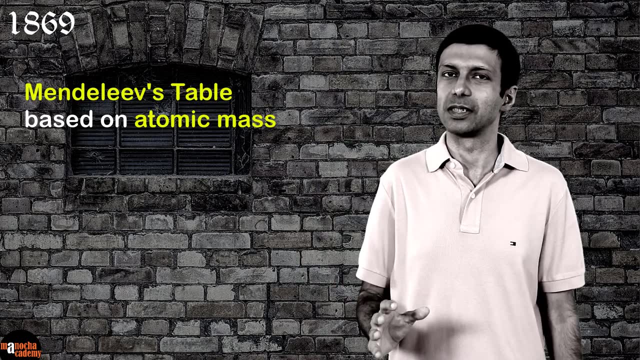 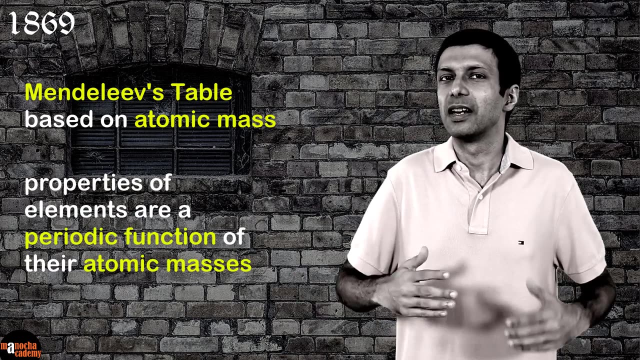 Till now all the classifications, including Mendeleev's, were based on atomic mass. So elements were arranged in the increasing order of atomic mass, And his periodic law stated That the properties of elements Are based on atomic mass, Are a periodic function of their atomic masses. 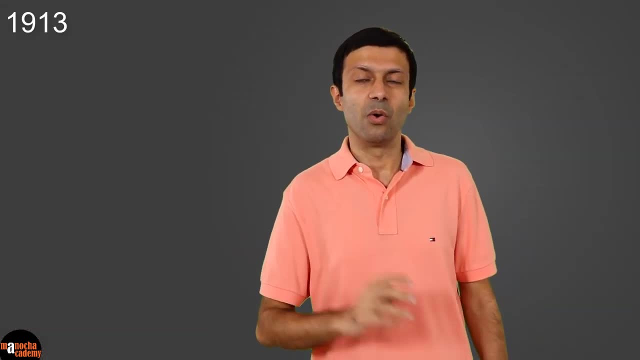 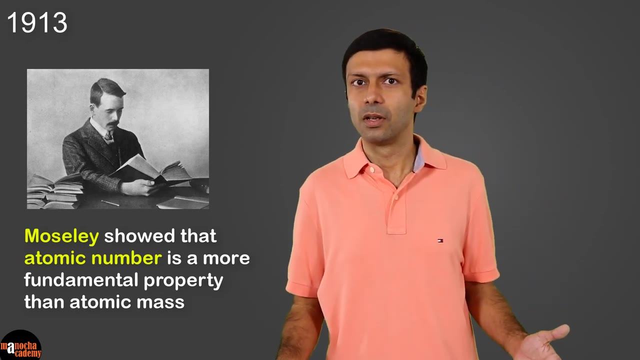 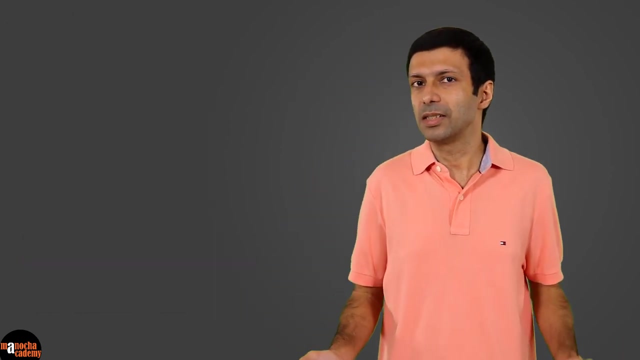 Now let's move ahead to 1913. Where Moseley showed that atomic number is a more fundamental property than atomic mass. So what's the difference between atomic mass and atomic number? Atomic mass, as we discussed, is the mass of a single atom of an element. 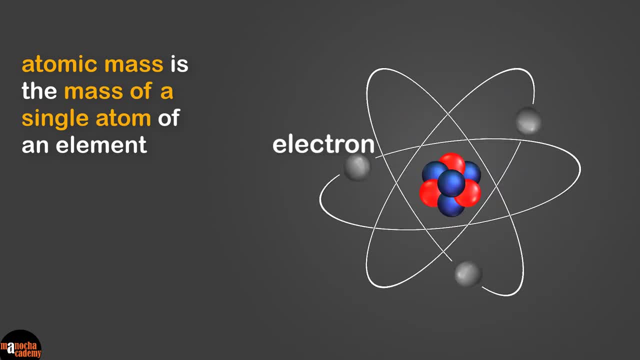 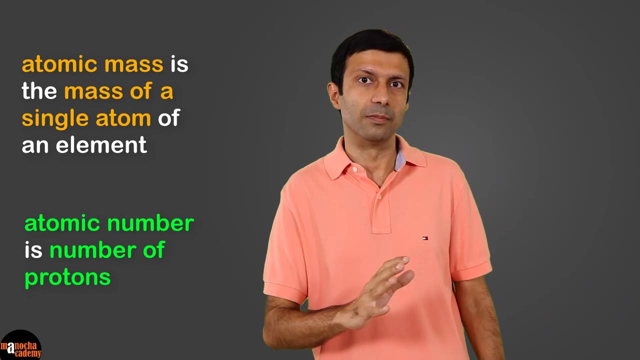 And with the discovery of subatomic particles Like electrons, protons and neutrons, Atomic number was defined as the number of protons present in the nucleus of an atom. So this was a complete shift And everything was now based on atomic number. 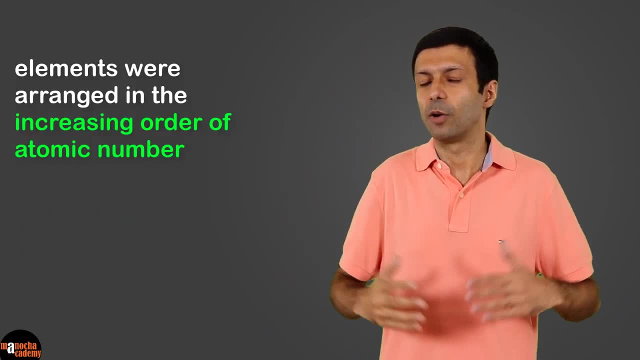 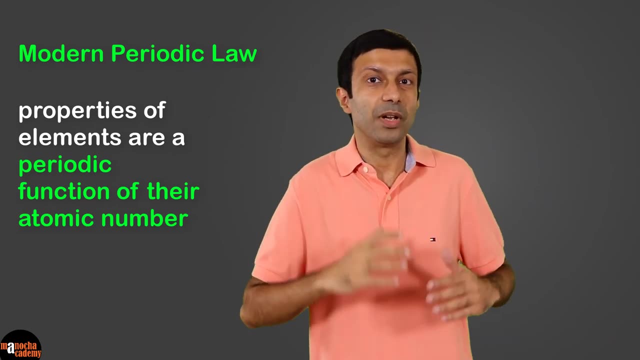 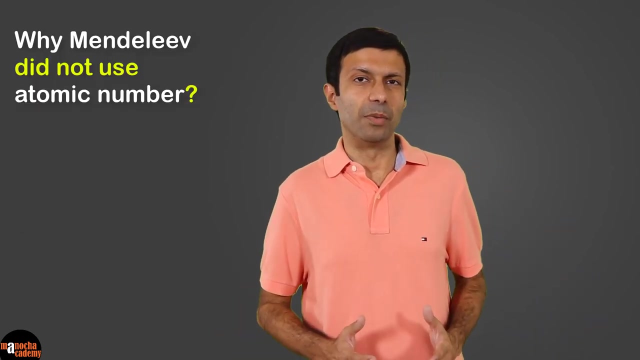 So elements were arranged in the increasing order of atomic number, And the modern periodic law stated that the properties of elements are a periodic function of their atomic number. You may be wondering: Why didn't Mendeleev use atomic number? Why was he using atomic mass?